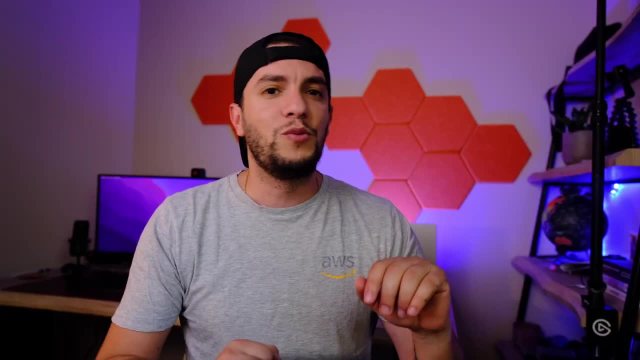 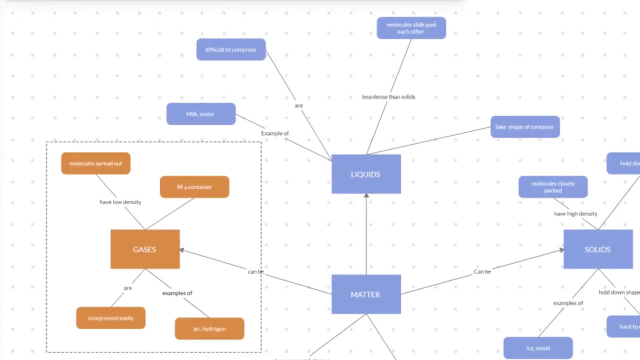 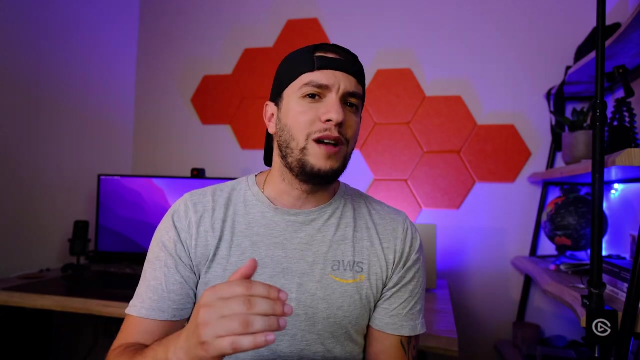 architecture diagram, But if you remember these tips we will talk about, you will start building them like a pro. You see, a diagram might look like a bunch of boxes and arrows, but it's much more than that. Knowing what every box stands for is not enough. The diagram should convey. 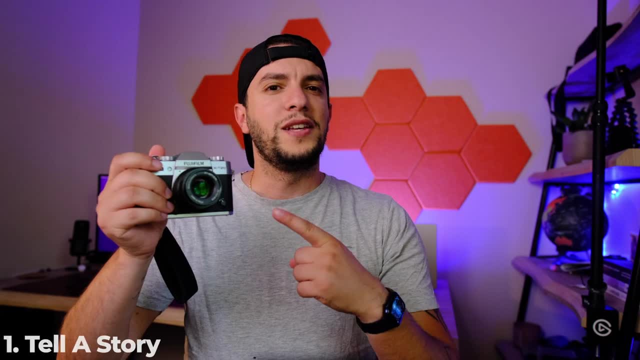 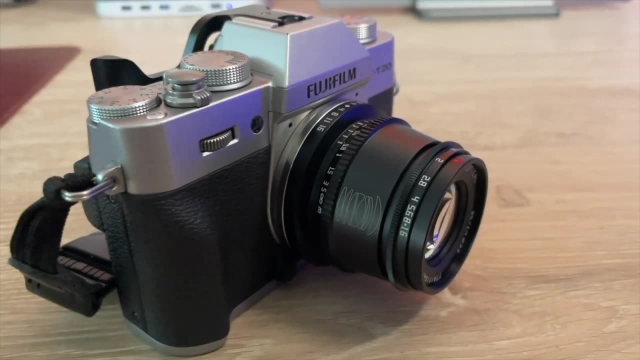 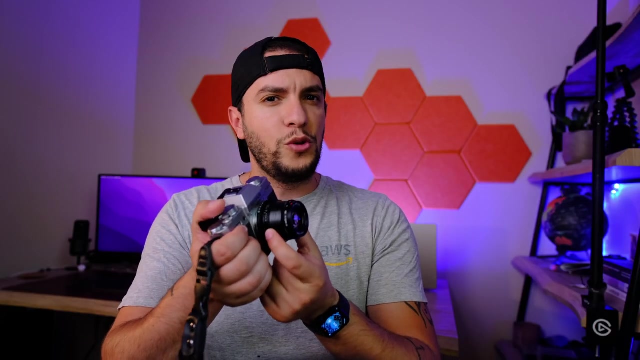 a message. It should tell a story. Let's take this Fuji x-T20, for example. It's a camera with buttons and dials and screens put according to a layout. I can know exactly what every button does- Here's the shutter button, Here's how to zoom- But does knowing the function of every button 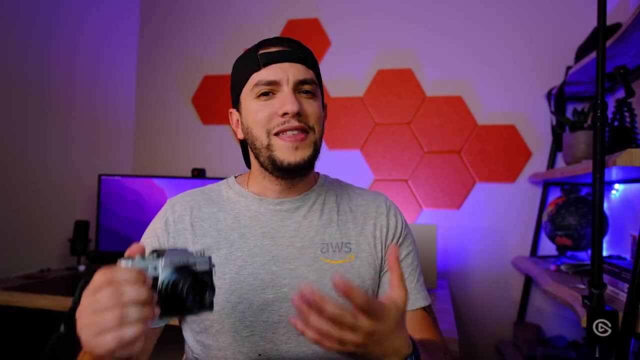 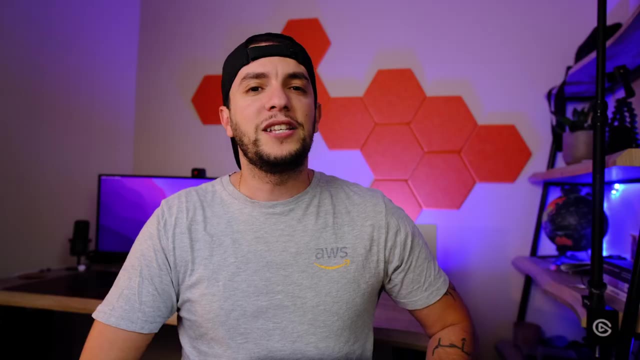 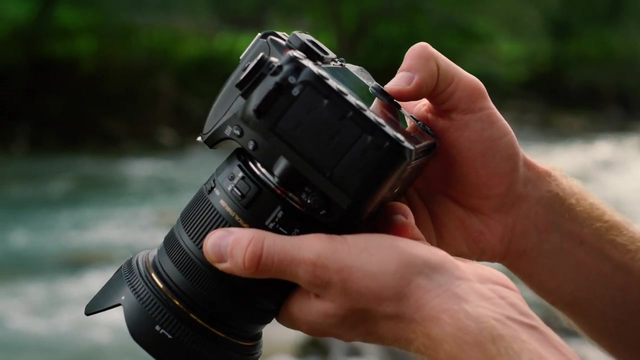 makes me a photographer? Obviously no, But the way these various components are ergonomically laid out helps me pick up on the underlying message, the message of how to properly take a picture. the ergonomic layout provides context and a deeper meaning than simply labeling the button of the camera, and that same concept applies when building. 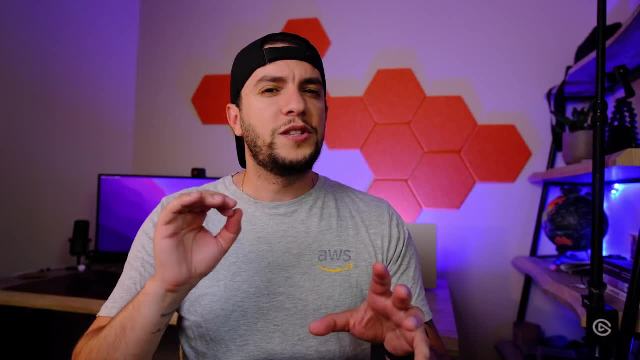 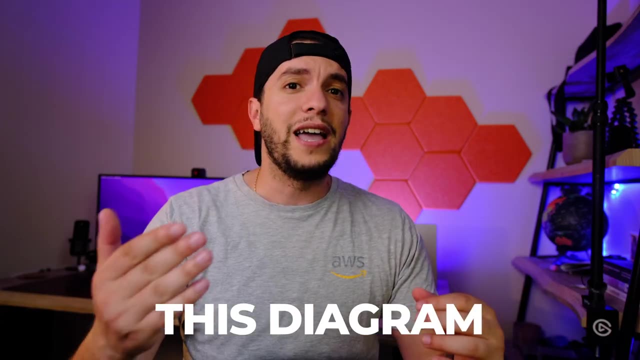 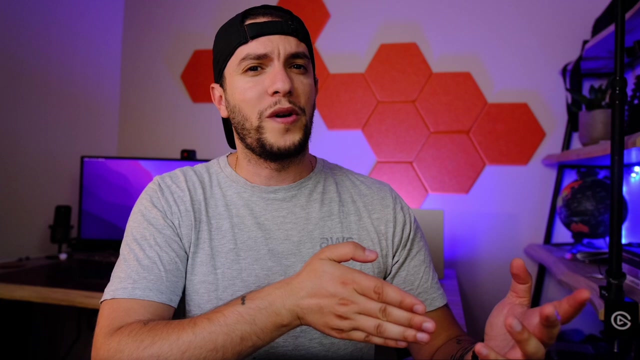 architecture diagrams. so, before you draw your first box on the page, figure out your message. if you don't know what your message is, well, ask yourself what is the value this diagram is providing? what is the story i'm trying to tell? am i doing a step-by-step migration story, a lift and 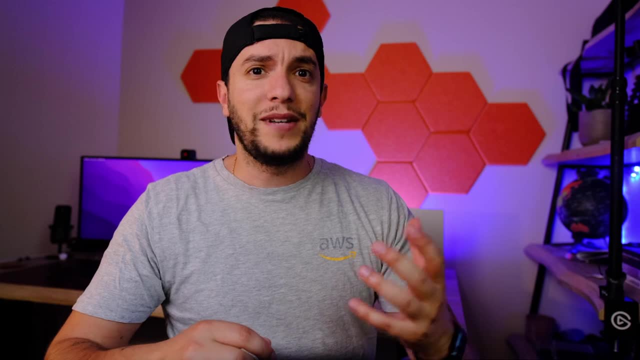 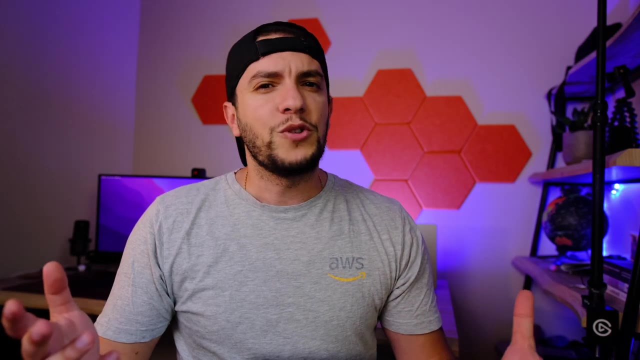 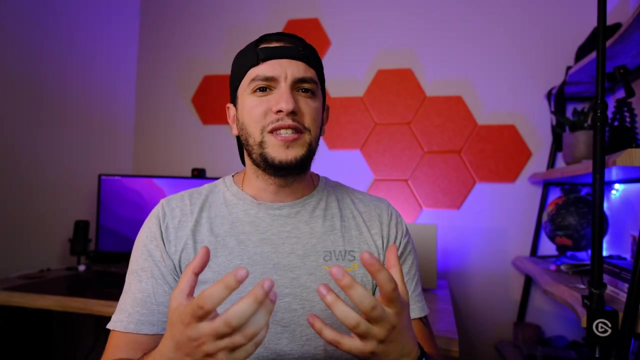 shift migration story. an etl extract: transform load story. if you're having a hard time telling the story, try to write it down. you know, just sometimes when you try to write down an explanation of what you're trying to accomplish and then you see written these words- well, you will have an easier time building your message. 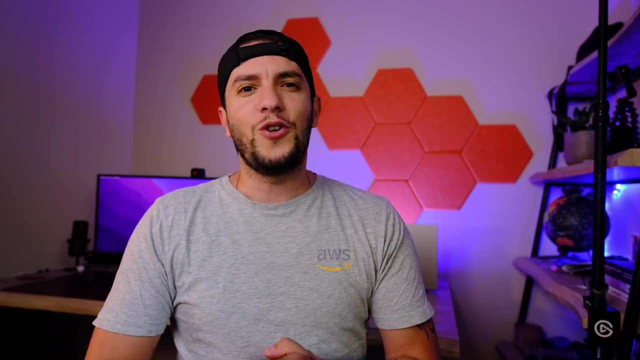 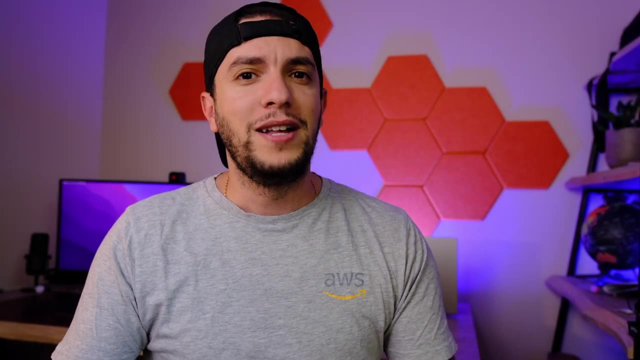 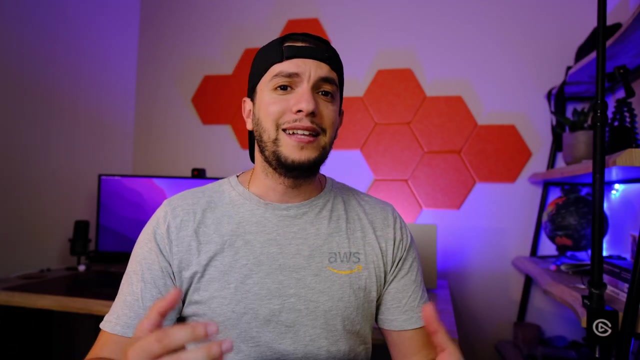 when i was learning my way to photography, the instructor on youtube didn't explain what every number, button, dial and handle did in the camera. that would have been overwhelming, you know, to say the least, and i would have retained nothing, knowing how my brain works. instead, they showed: 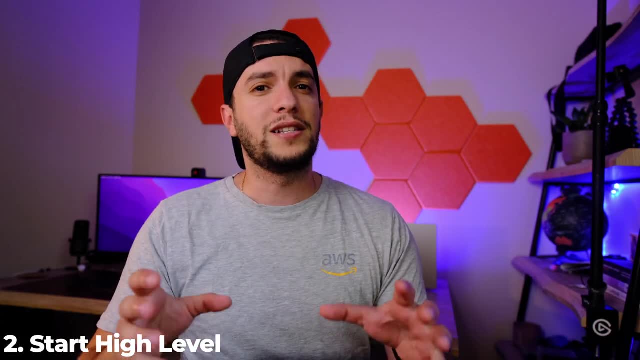 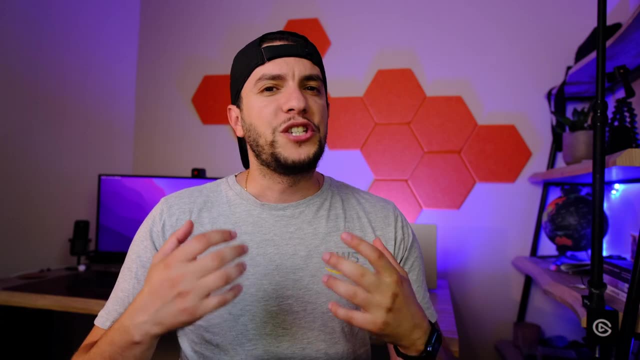 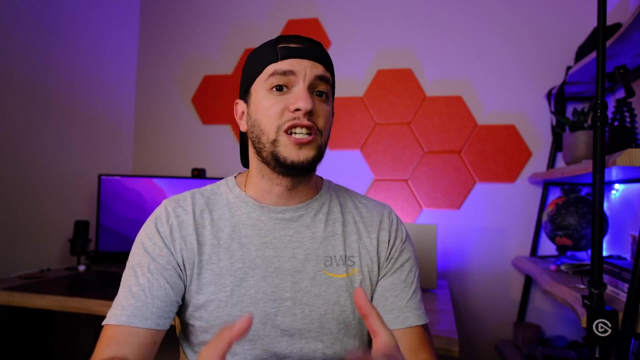 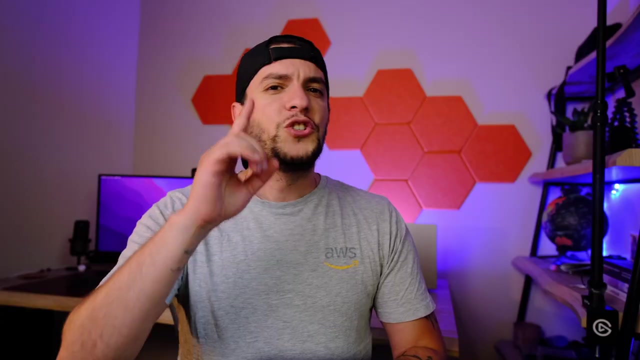 the necessary pieces to get comfortable with the concept of photography. as software engineers, we assume the more information the better, and we try to pack in information in data dense diagrams. but introducing your audience to something without the knowledge you have leaves your diagram looks like hieroglyphics. so ask yourself the following questions: who is the? 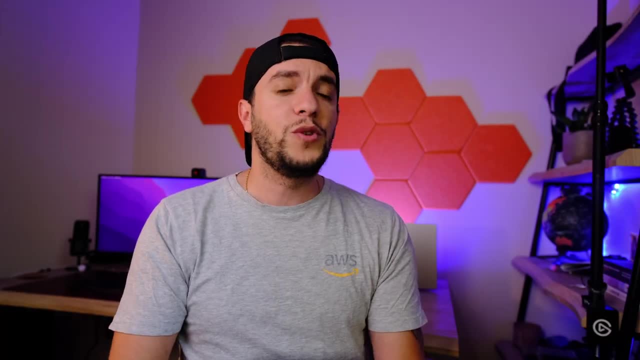 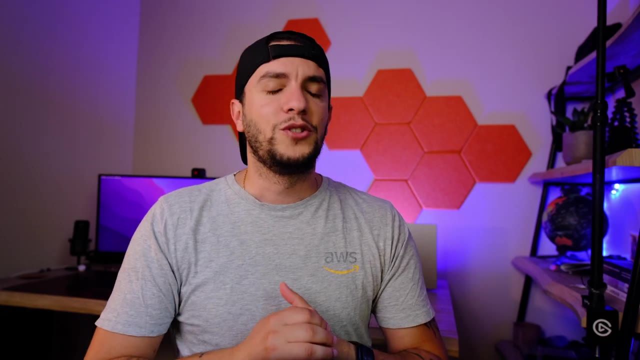 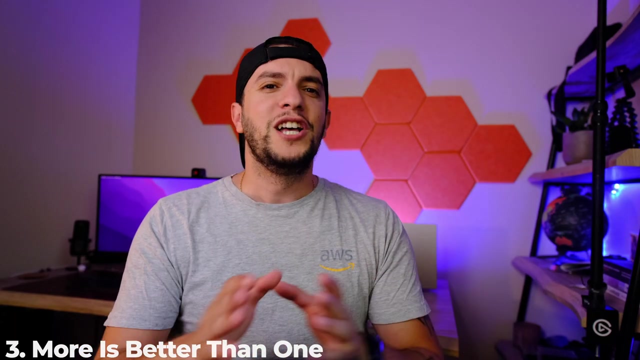 intended audience of this diagram? are they familiar with your domain? are they a developer who understand all these technical details and then adapt your diagram to the audience, which brings us to the next step. more is better than one. we're telling a story, remember, so have your first diagram sitting: the stage building. 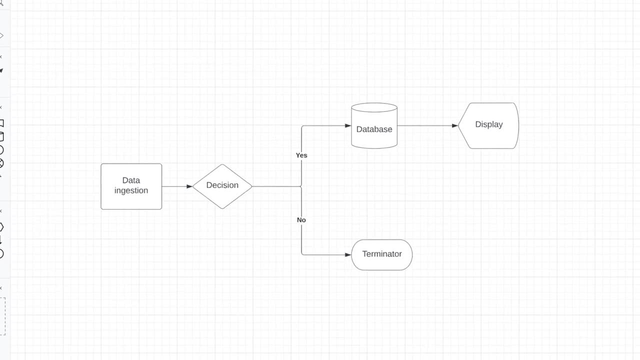 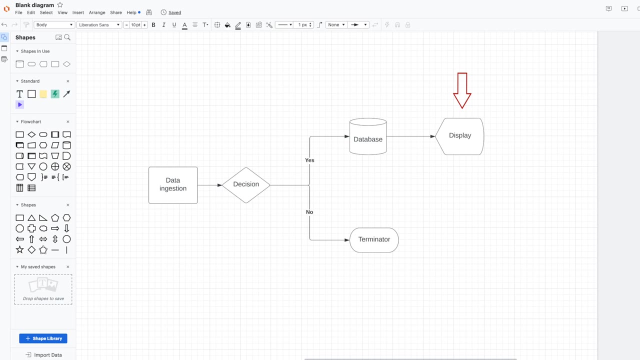 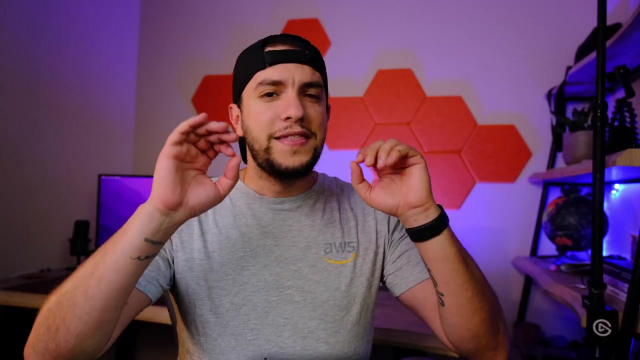 up context, building up common and shared understanding with your audience. but once you start presenting, you will likely get a handful of questions: how does this component interact with the main database? how will this component be secured? where do i transform this message? and then- And that's where your second, your third or your fourth diagram come into play- 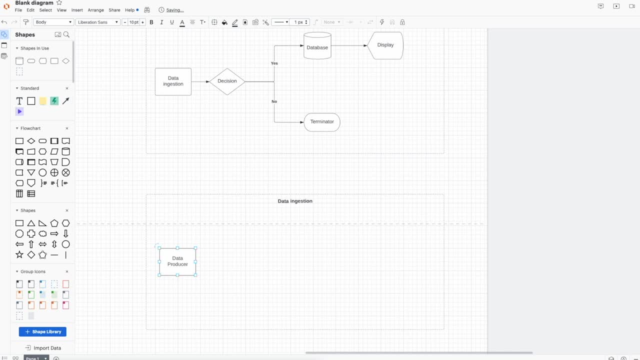 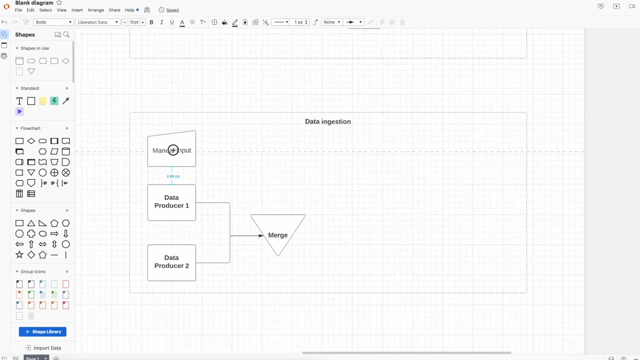 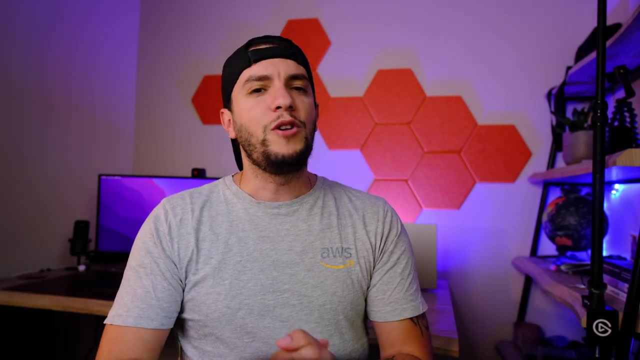 Think of them as companion diagrams that make your story significantly more impactful and easier to understand. You can answer security questions with a specific diagram that shows the authentication mechanisms, encryption solution, data flow and whatnot. Now, going back to the camera analogy, this is where you start learning about prime versus. 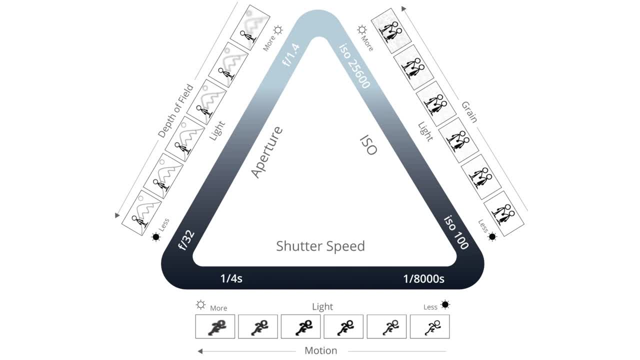 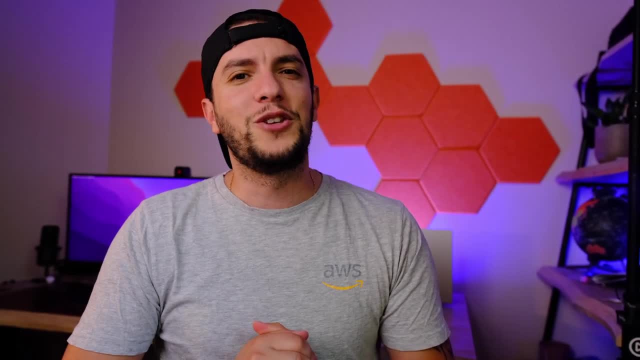 zoom lenses, the various focal lengths, the exposure triangle. These are not necessary for taking a picture, but you'll learn pretty quickly that they are needed if you want to be or become a photographer. All right, two more tips to go, but before that, if you're new to the channel, hi my. 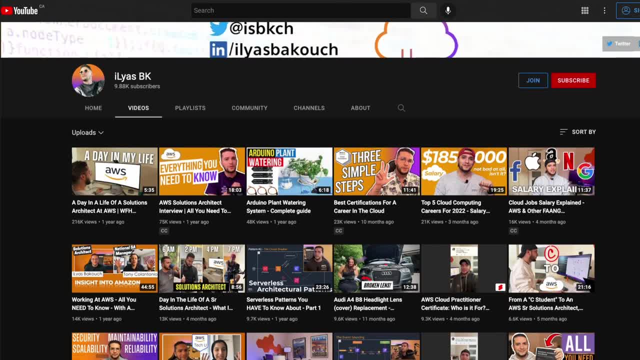 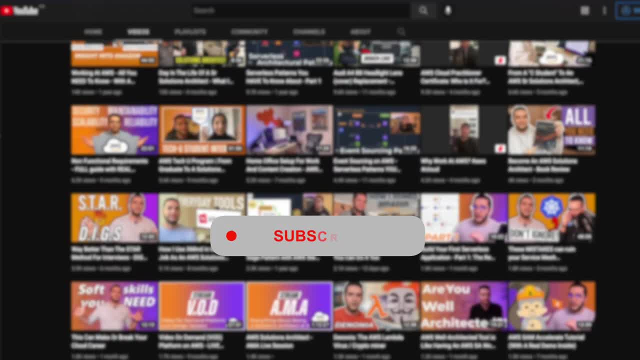 name is Ilyas Nice to meet you. This channel is all about getting to the cloud and growing in the cloud, you know, career-wise, but also from an architectural point, technical point. If you like what you see, make sure to hit the subscribe and notification bell. 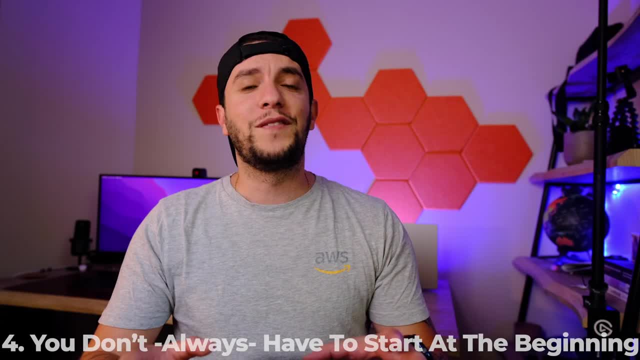 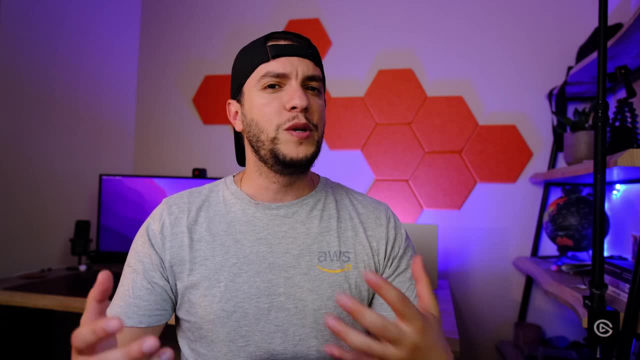 So you don't miss out on new uploads. You don't always have to start at the beginning. Now that you know your audience and the level of familiarity with your domain, you can probably skip a few components and jump ahead in your presentation. So you don't bore them with stuff they already know. 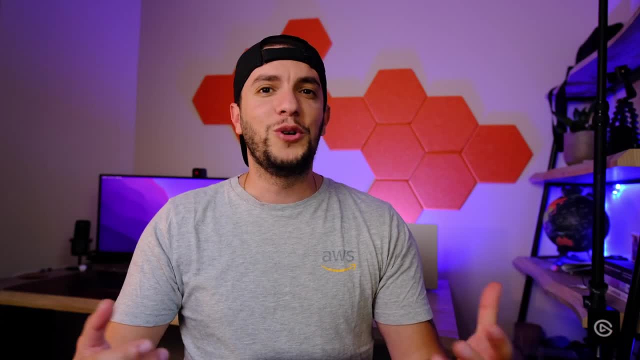 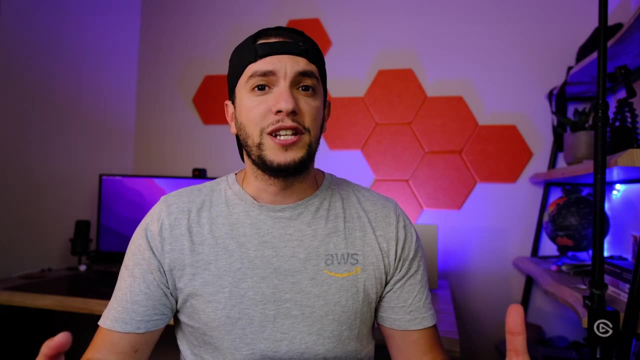 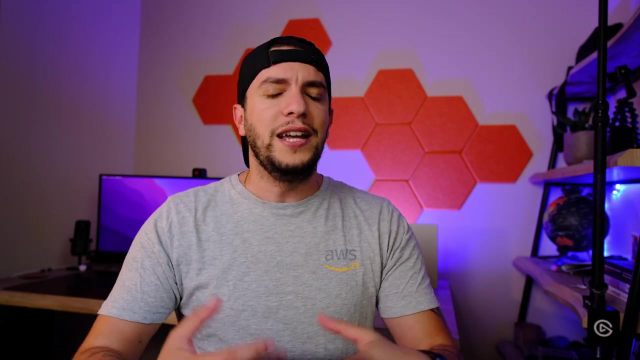 I'm going to go back to my camera again. It's safe to assume that in 2022, everyone is familiar with what a JPEG is, So no need to explain that in depth. or if you were teaching someone to drive a manual transmission, you wouldn't show them the steering wheel, gas pedal and brake pedal.